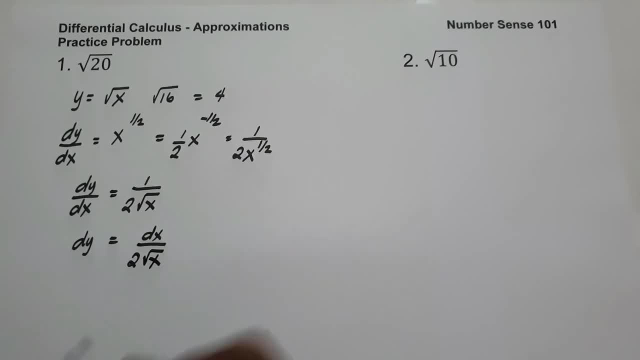 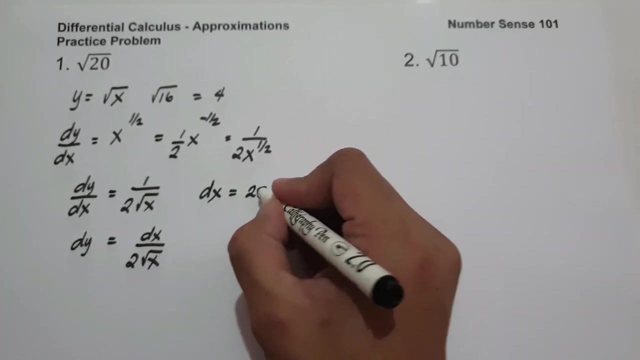 over two square root of x. And then let us find the value of drugs, DX. that is the change that we use in our equation. So all you have to do to find the value of dx, Let us have the. dx is equal to twenty minus sixteen. 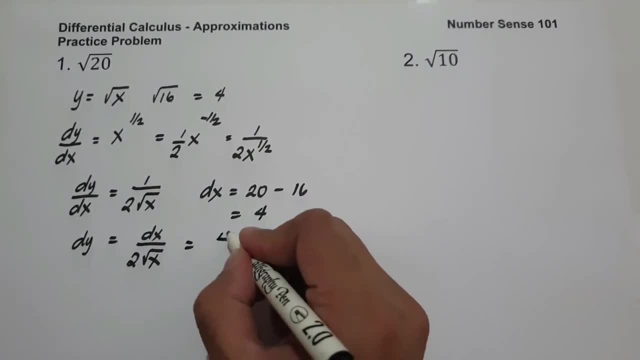 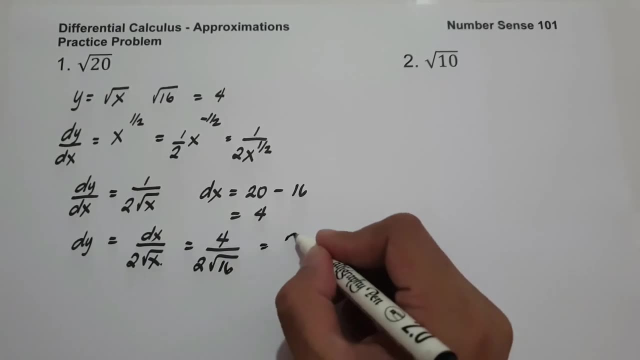 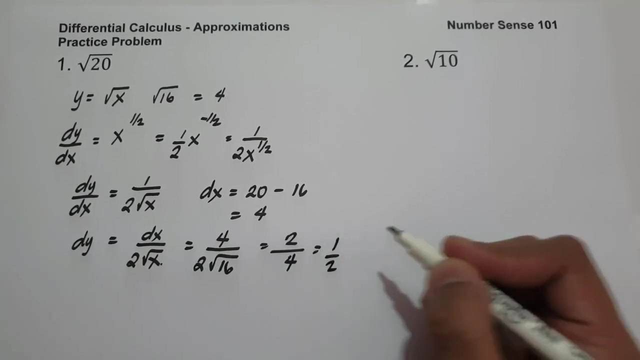 and that is four. Therefore we have four over two. square root of x, that is 16.. Four, divide by three is 16.. 2, that is 2, and then square root of 16, that is 4. so therefore it will give us 1 half. so if you write, 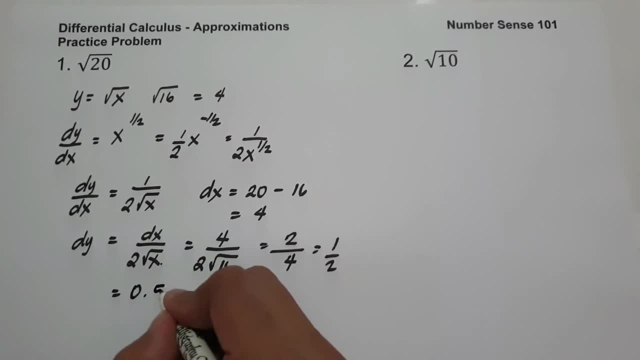 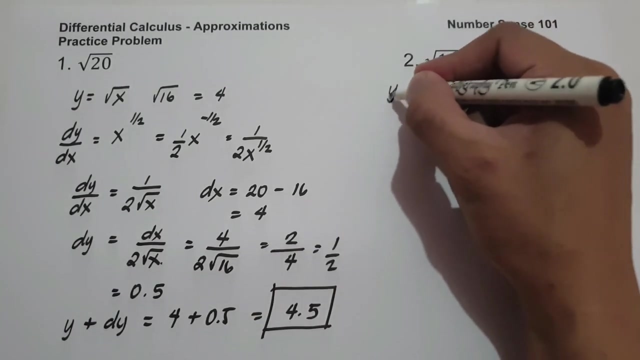 1, half into decimal, that is 0.5. so therefore let us have y plus dy, so the approximate of square root of 20, that is 4 plus 0.5, that is 4.5, and this will be our answer on number 2. we have square root of 10, so let us have: y is equal to square root of x. 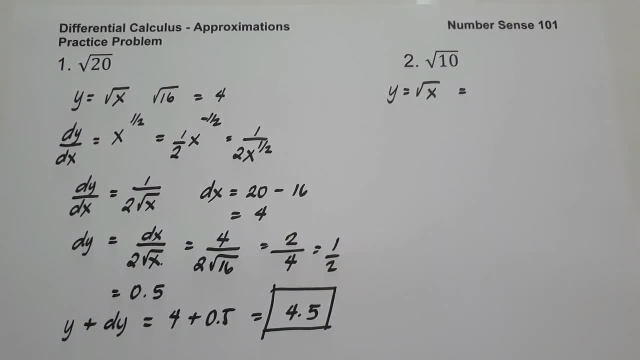 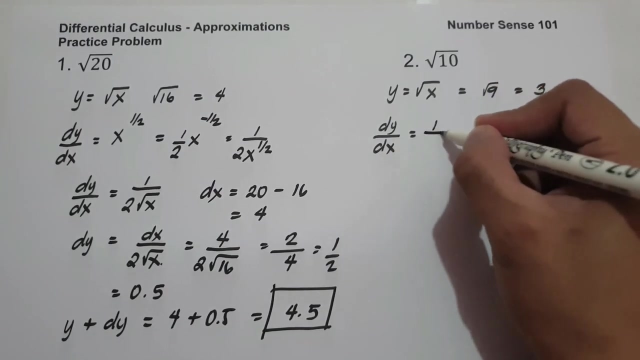 and we are going to think of perfect square closer to square root of 10, and that is square root of 9, and square root of 10 is square root of 9, and square root of 10 is square root of 9 of 9, that is 3. so let us differentiate this one. this will be: dy over dx is equal to 1 over 2. 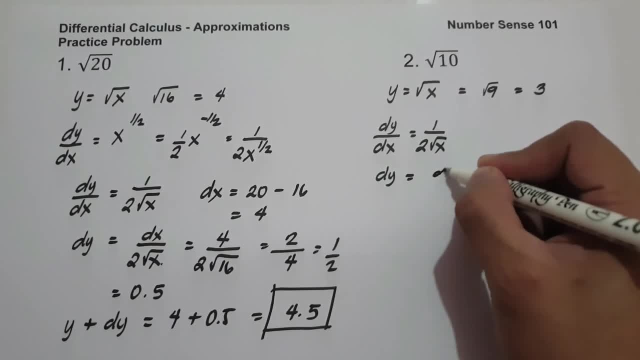 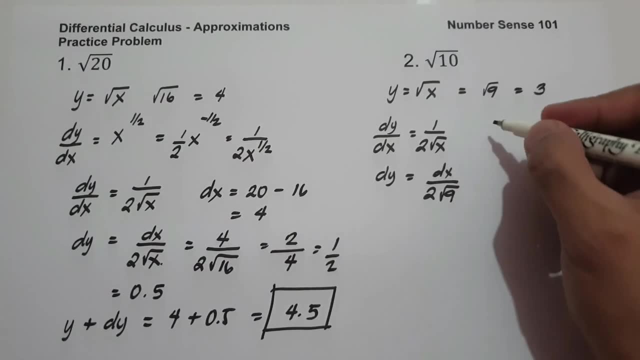 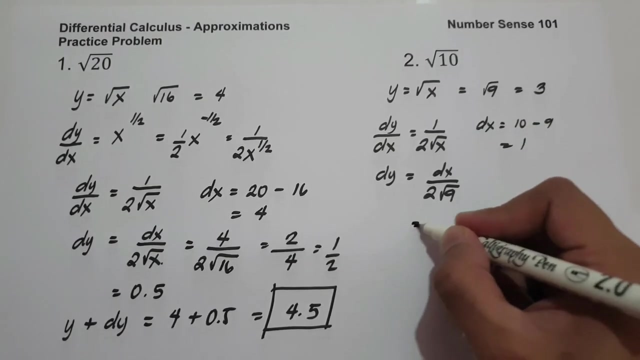 square root of x or dy is equal to dx over 2 square root of 9, and the value of dx, that is dx, is 10 minus 9, that is 1. so it will give us 1 half square root of 9, that is 3. so this will be. 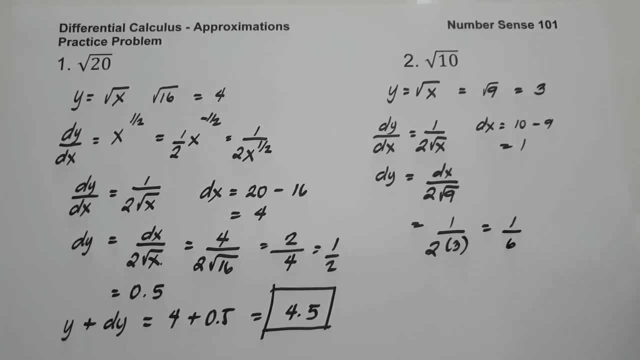 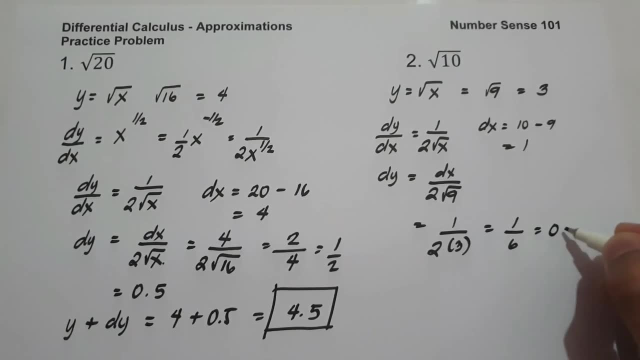 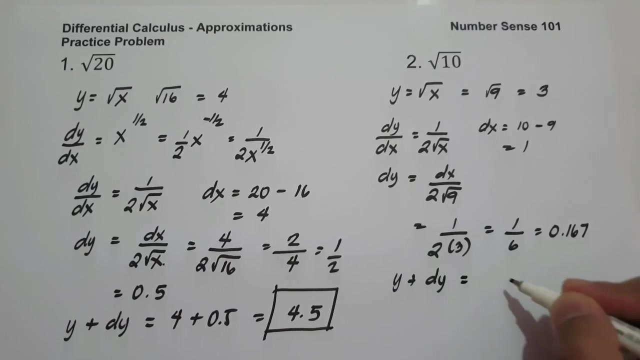 1 over 6 and if you are going to divide 1 over 6, it will give us 0.167. therefore, y plus dy, that is 0.167, 3 plus 0.167, that is 3.167, and this will be our answer. 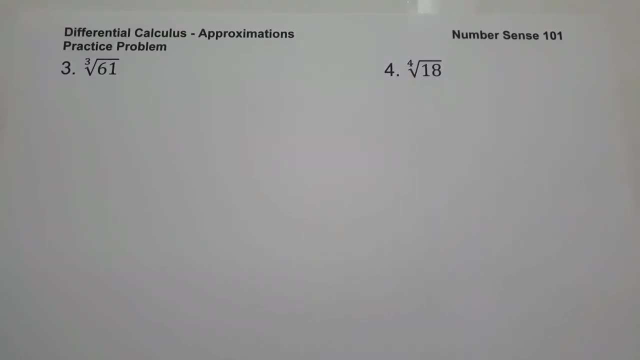 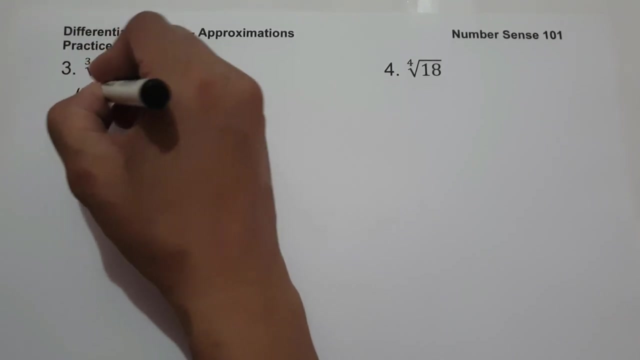 on number three, how can we find the approximate value of cube root of 61? so the first step that we're going to do is to express this one in terms of y and let us represent 61 as x, and that is, y equals cube root of x. 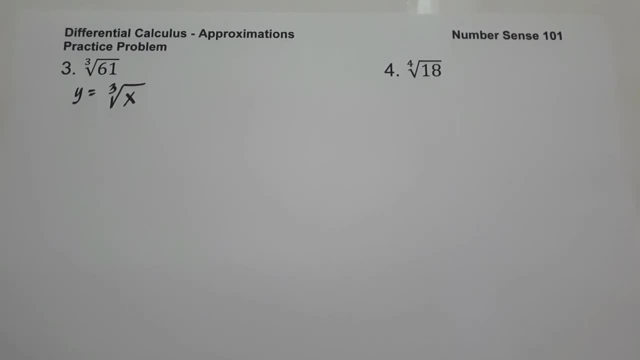 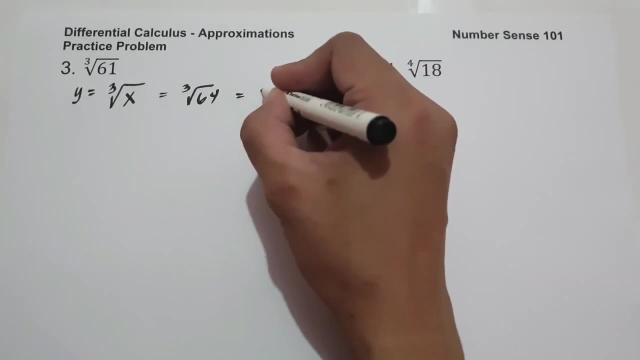 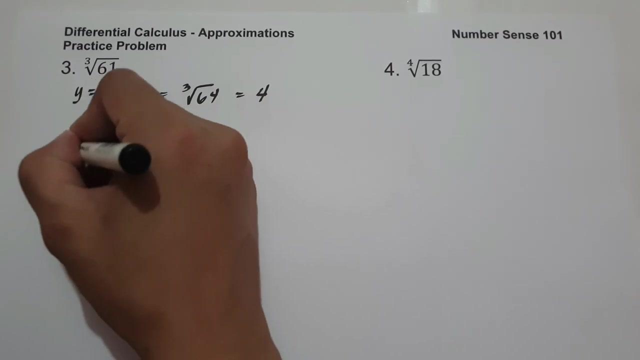 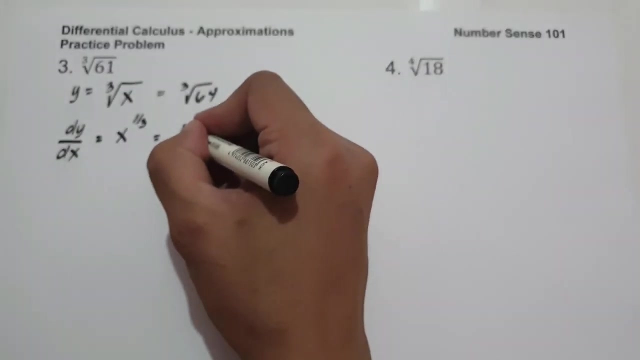 and we are going to think a perfect cube closer to cube root of 61, and that is cube root of 64, and cube root of 64, that is 4. and then let us differentiate this one, that is dy, over dx, and let us write x raised to one-third. so let us differentiate x raised to one-third, that is one-third. 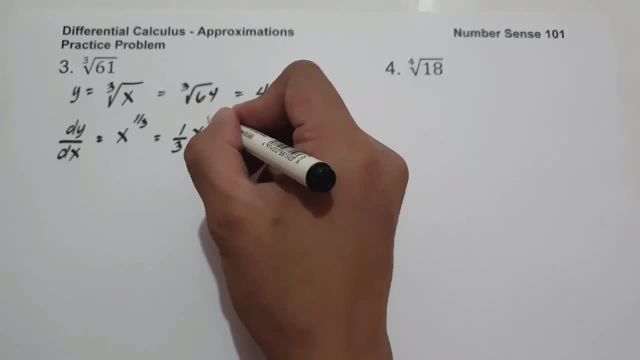 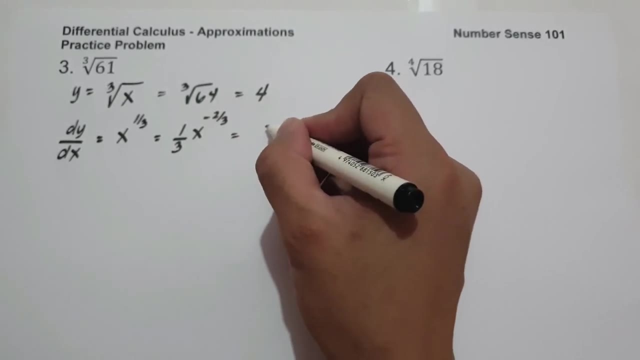 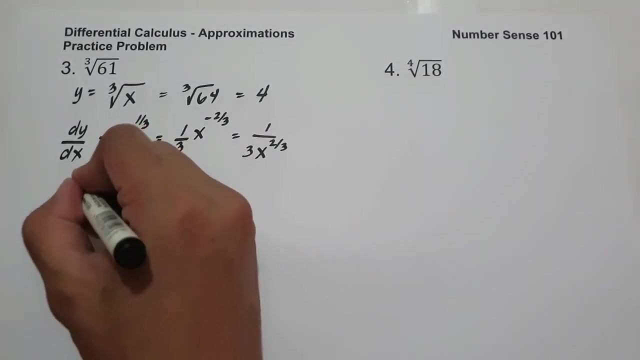 x one-third minus one, that is negative two-third. and to eliminate the negative sign on the exponent, let us write x into the denominator, that is 1 over 3, x raised to positive two-third, and that is dy over dx is 1 over 3, and let us 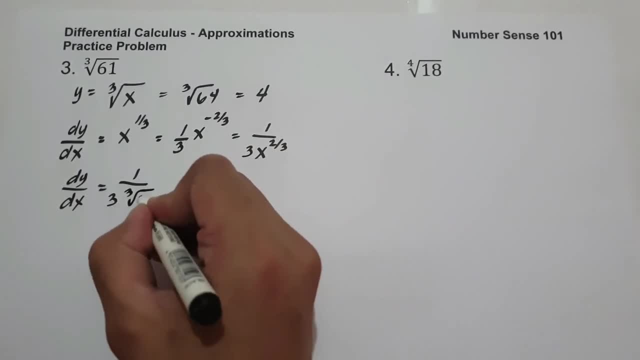 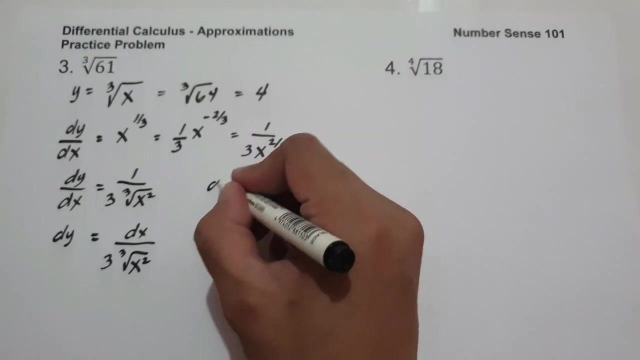 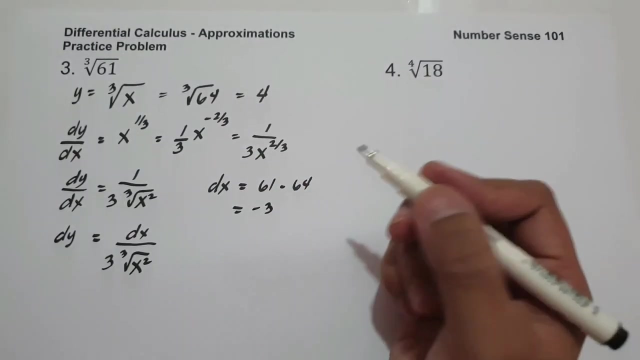 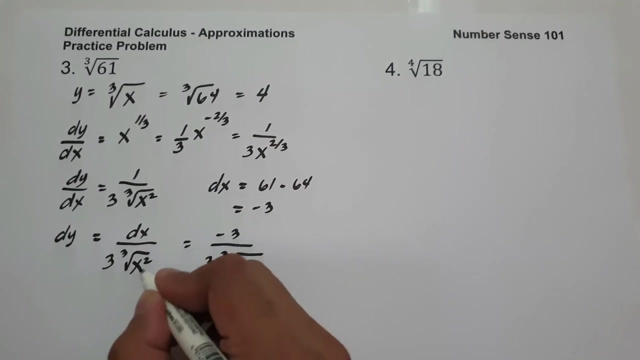 write x, raised to two-third, as cube root of x square and then let us have dy, that is x over 3 cube root of x square, and let us find the value of dx, that is 61 minus 64, and that is negative 3. it will give us negative 3 over 3 cube root of x square. that is the value of x, that is. 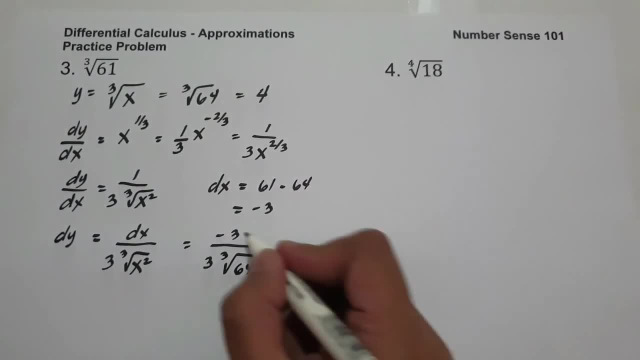 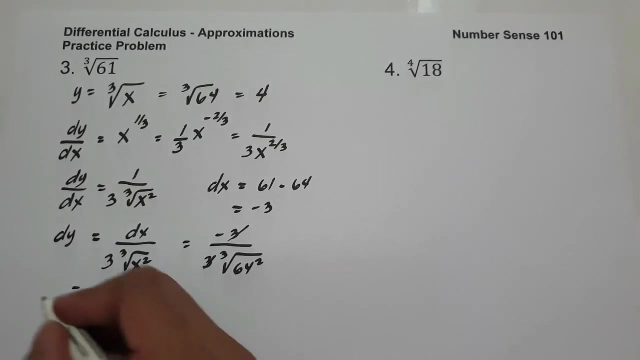 64 and then square, so let us cancel this one. it will give us negative 1 over cubo to 64, that is 4, and then 4 square, that is 16. therefore the value of ty is negative 1 over 16. and to find approximate value of cube root of 61, let us have y plus the y, that is 4. 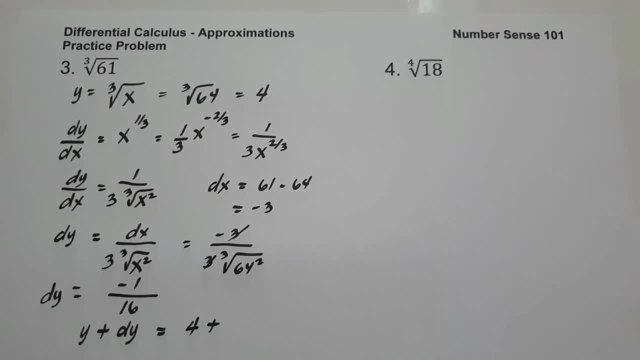 plus 1 over 16 and to simplify, let us have 16 multiplied by 4. that is 64 minus 1 over 16 and that is 63 over 16.. If you're going to divide 63 over 16, it will give us. 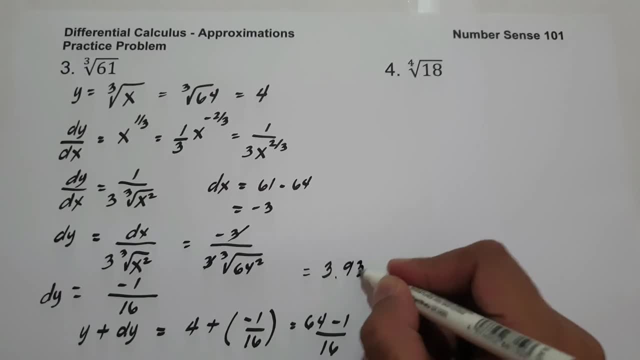 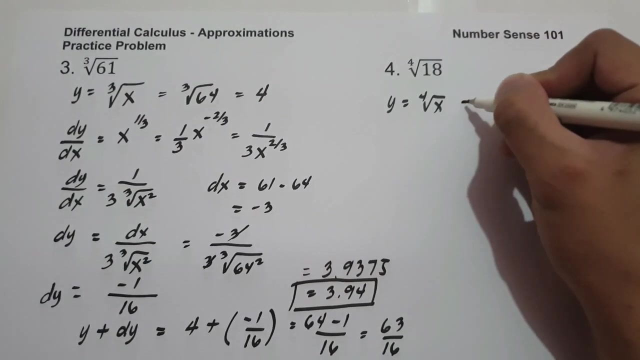 3.9375, or you can write as 3.94 and this will be our answer. What about number four? How can we find the approximate value of fourth root of 18?? So let us have y equals fourth root of x and we are going to think a perfect fourth root closer. 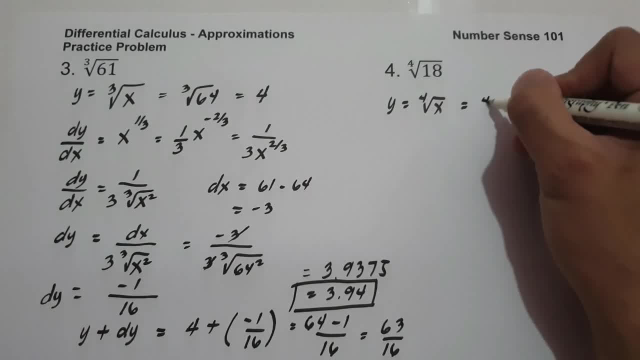 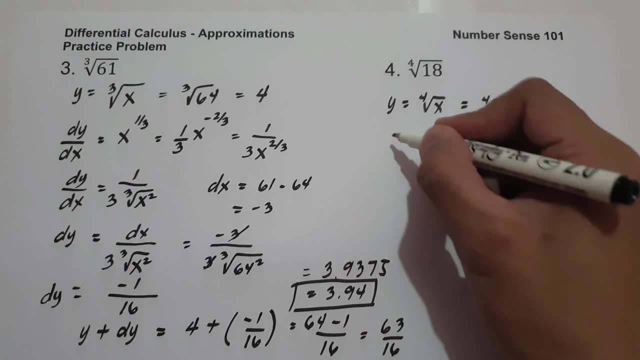 to fourth root of 18, and that is 3.9375.. So let us write as 3.9375, and this will be our answer: Fourth root of 16.. Fourth root of 16, that is 2, and let us differentiate this one. This is: 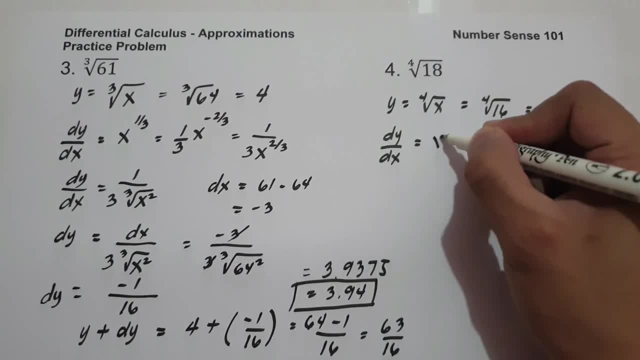 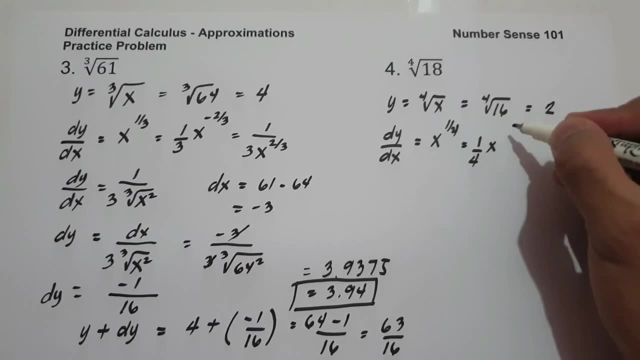 dy over dx is equal to x raised to 1 fourth, It will give us 1 fourth x 1 fourth minus 1, that is negative 3 over 4. and to eliminate the negative sign, that is 1 over 4- x raised to positive 3 over. 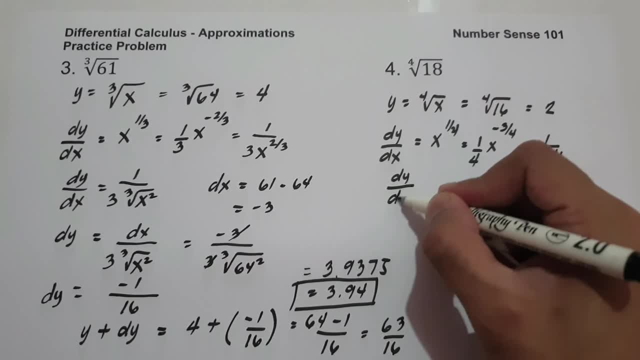 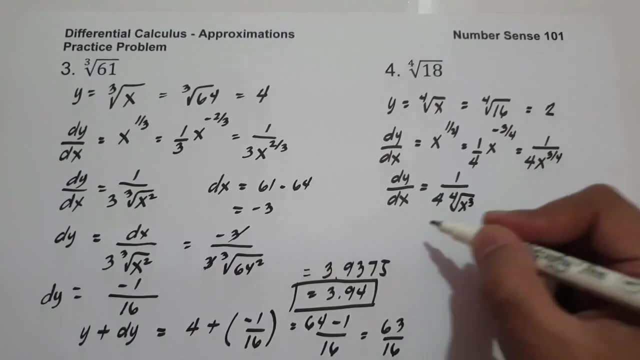 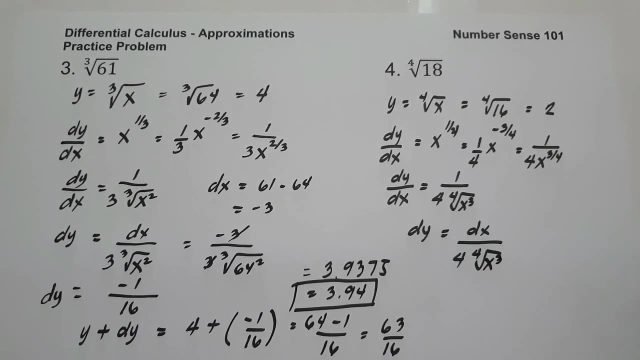 4. So you can have dy over dx, 1 over 4 fourth root of x cube. So let us have: dy is equal to dx over 4 fourth root of x cube, and then let us have dx, that is 18 minus 16, that is 2, and this will be. 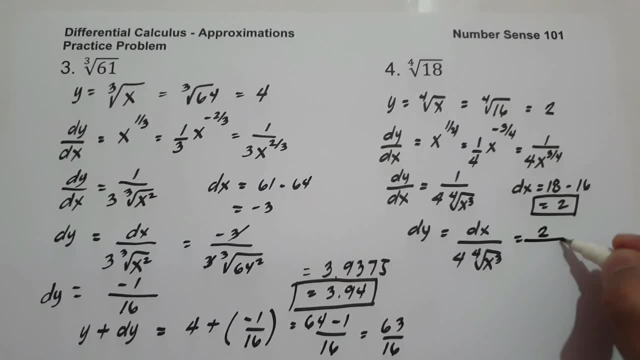 the value of dx. So let us have 2 over 4, fourth root of x, cube, and then let us have dx, that is 16 raised to 3.. So let us cancel this one. It will give us 1 over 2 and fourth root of 16, that is 2. 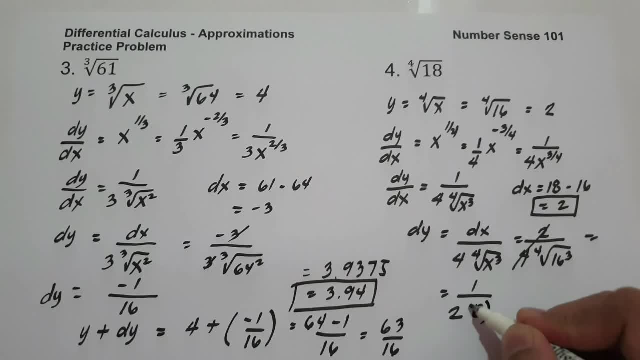 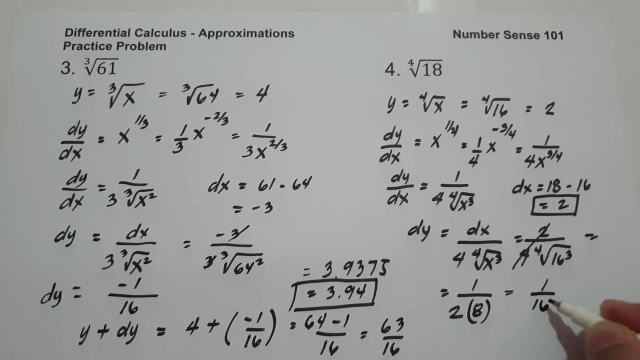 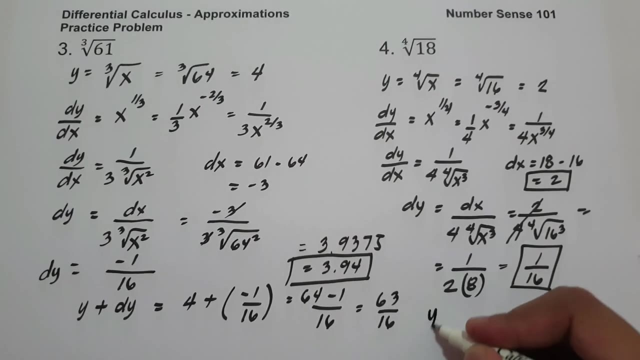 and 2 raised to 3, that is 8.. So let us have 1 over 2 times 8, that is 16, and this will be the value of dy. So let us have y plus dy, that is 2 plus 1 over 16, that is 2 and 1 over 16. or you can write as 16 times 2, that is 32 plus.